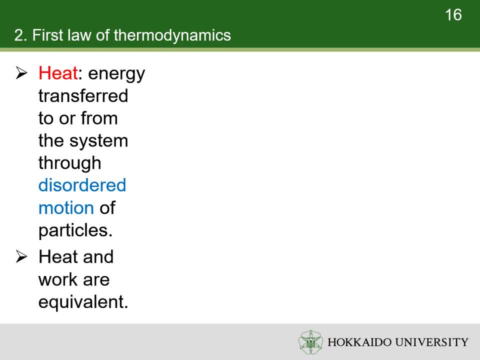 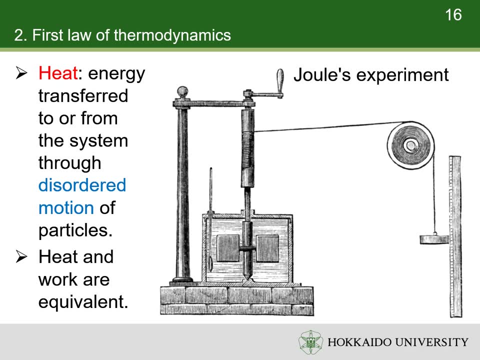 more violent. The equivalency of heat and work was proved by a series of experiments. The most famous one is James Prescott Joule's experiment. In Joule's experiment, gravity does the mechanical work on a falling weight. A paddle wheel was driven by the falling weight in an isolated 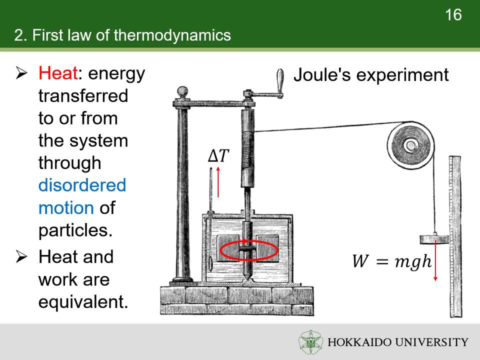 barrel of water, The temperature of the water increases When the water stopped swirling. the temperature increase is proportional to the work done, to the weight. So doing work to a system is equivalent to heating it. In Joule's experiment, the ordered the motion of water caused by the spinning paddle. 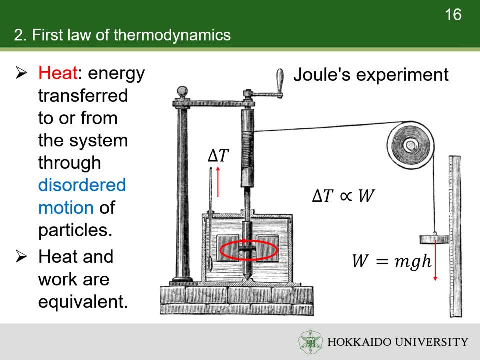 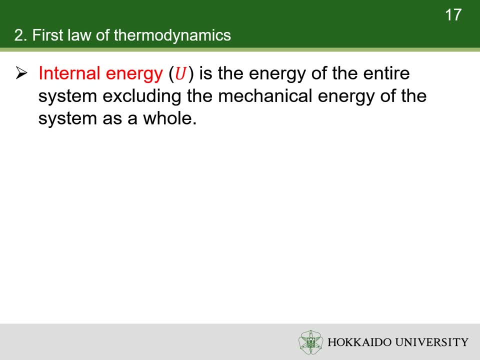 wheel gradually converts to disordered motion of water molecules due to the viscosity of water. Internal energy is the energy of the entire system, excluding the mechanical energies of the system as a whole. For example, the gravitational potential energy of the whole system is excluded from the internal energy. The kinetic energy of the whole system is: 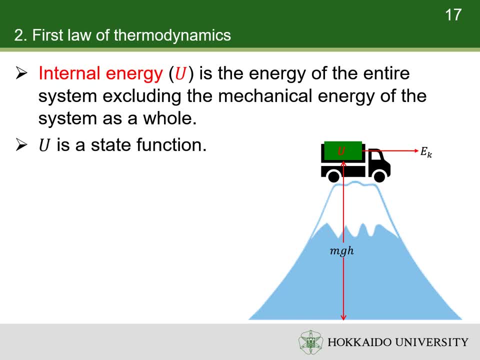 also excluded. Internal energy is a state function. For example, the不行 energy ut is excluded from the internal energy. The kinetic energy ut is also excluded from the whole systemTHE WAVY ENERGY OF THE ENTIRE SYSTEM EXCLUDES THE ACTO. CAN hj T ochai Hke. 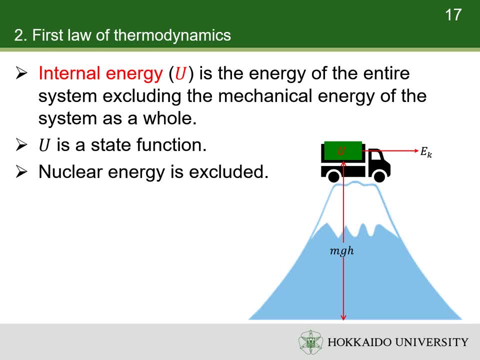 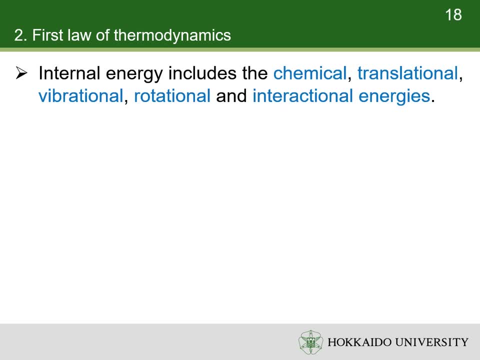 In chemistry we don't consider the energy caused by nuclear interaction as well, that is, the nuclear energy. In chemistry, the internal energy includes chemical energy stored in chemical bonds and kinetic and potential energy of the atoms. For example, the vibration of atoms in molecules store potential and kinetic energy. 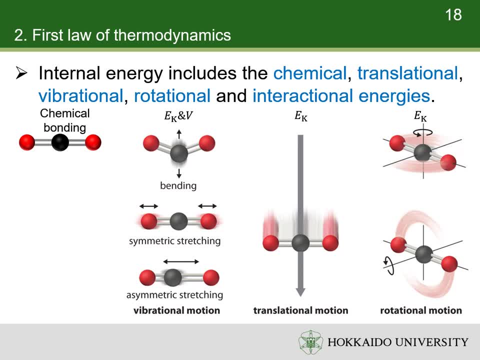 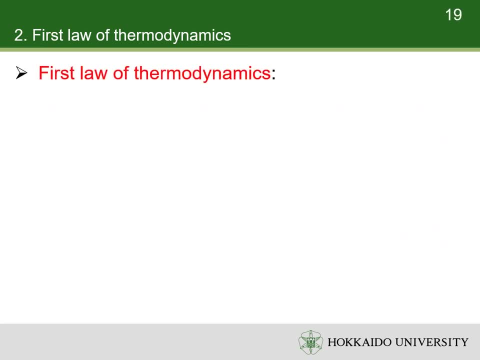 The rotation and translation of molecules store kinetic energy. The interactions between molecules stores potential energy. The first law of thermodynamics states that the change of internal energy is the sum of heat and work. The first law of thermodynamics is a version of law of conservation of energy. 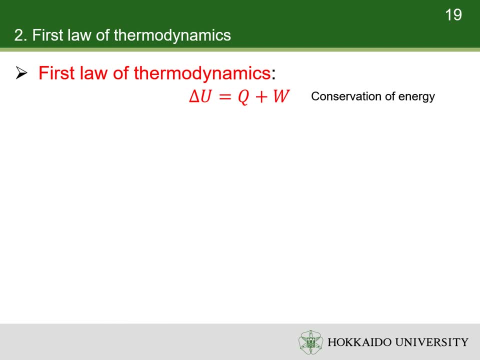 For a closed system, the energy change is equal to the net energy flow into it. For example, if a system receives 150 joules heat from its surroundings and it does 10 joules work to the surroundings, the change of its internal energy is 140 joules. 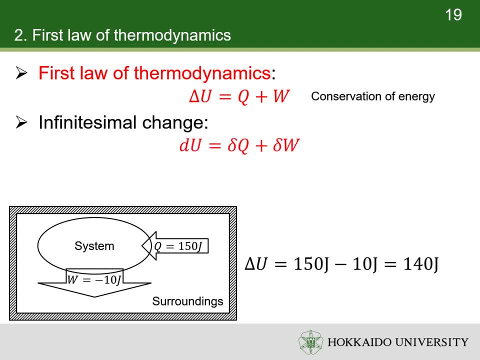 If the change is infinitesimal. the first law of thermodynamics states that the change of internal energy is the sum of heat and work. The second law of thermodynamics can be written in infinitesimal form If there is no work other than PV work. it is in the following form: